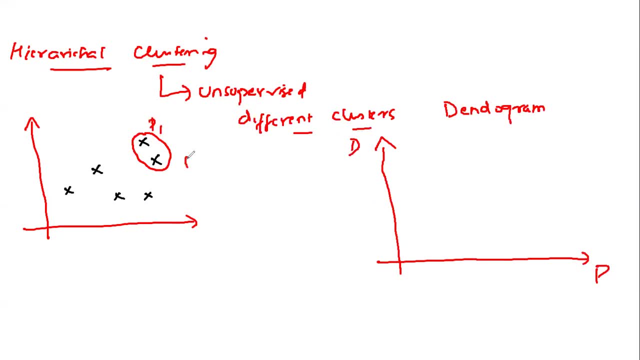 Now, if I am considering these two points and I name it as P1 and P2, suppose, if I draw P1 and P2 and suppose the distance between this is 0.5.. What I'm going to do is that I'm going to combine this and this will be 0.5. 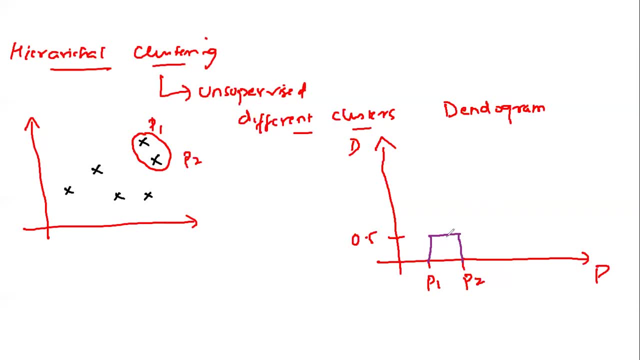 So this is one type of dendogram that we have created for P1 and P2.. Then after that we'll try to find out the distance between this cluster and this point and try to find out which are the next nearest point, And from that I found out that these two are the nearest point. 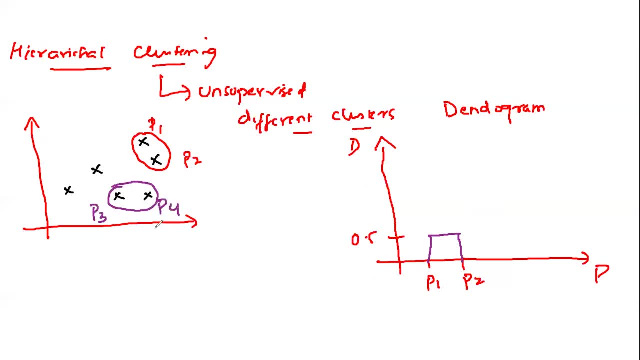 And here I get specific points And here I get specify this as P3 and P4.. So what I'm going to do is that I'm going to define another point that is P3 and P4. And suppose this distance is somewhere around 1.. 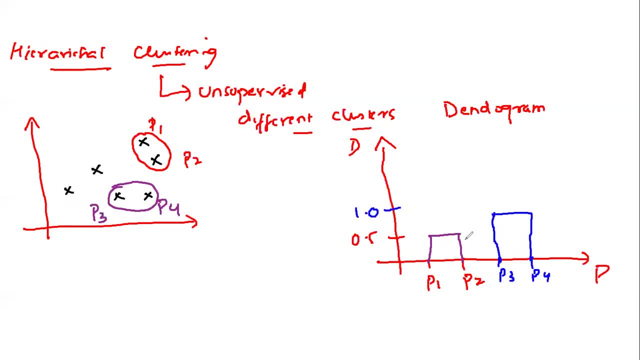 So I'm going to combine this and this distance will be 1.. Now, currently I've got two groups. Still they are points, And this again we have found out that these are the next nearest point, So suppose I make it as P5, P6. 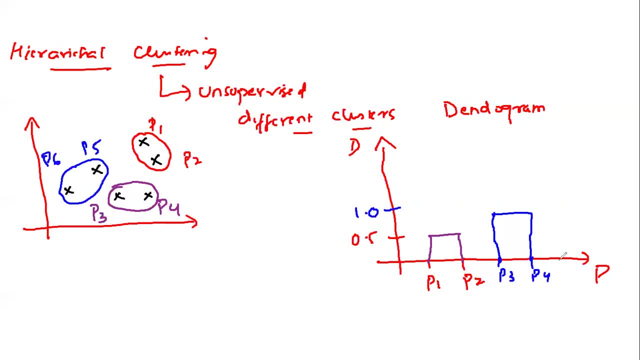 Then again I will be having something like this: P5 and P6.. Suppose I calculate the distance somewhere here. It is coming around 1.5. Suppose this is 1.5.. I have combined this. Then, finally, I'll try to find out which will be the nearest clusters to this. 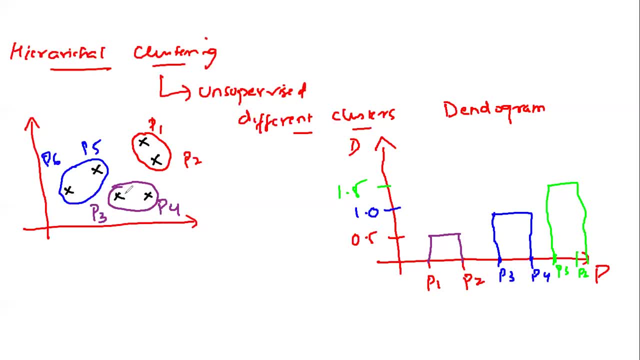 And suppose I found out that these two clusters are very, very near. So what I'm going to do, I'm going to combine these two clusters where I have points like P3, P4,, P5, P6. And I can combine this together like this, where my distance is actually 2.. 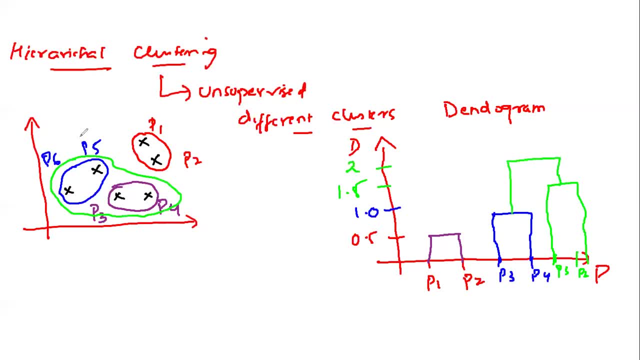 Finally, I'll combine this whole group as one cluster where I'll include P1 and P2, because these are my next nearest one. Suppose this is 2.5.. This P1 and P2 will get connected here. So this is how my dendrogram looks like, right? 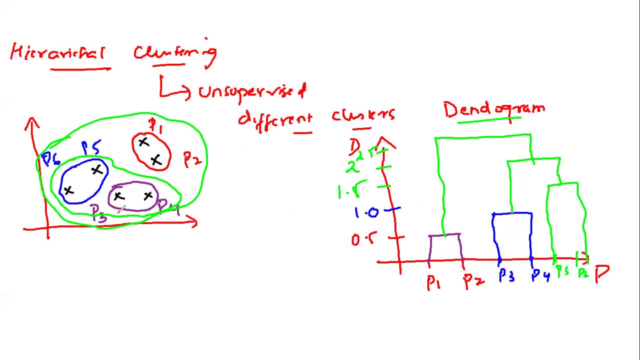 But what is the main aim? Just remember, guys, this is an unsupervised machine learning technique And our main aim is to basically find out that what should be the exact number of clusters should I use in order to classify my point properly? Not classify. 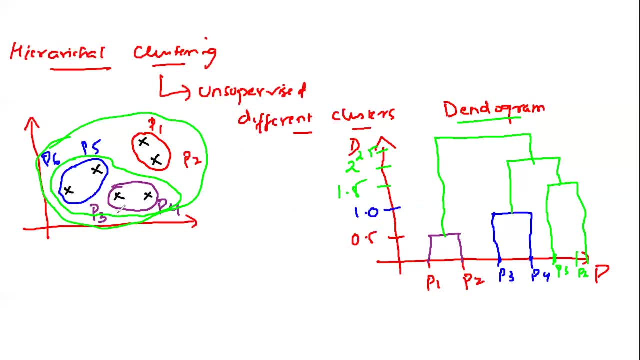 Instead group my points properly. Clustering works basically on the similarity of the data. right. Similarity of the data is basically that we are calculating over here with respect to the distance, And this distance is measured by something called as Euclidean distance. 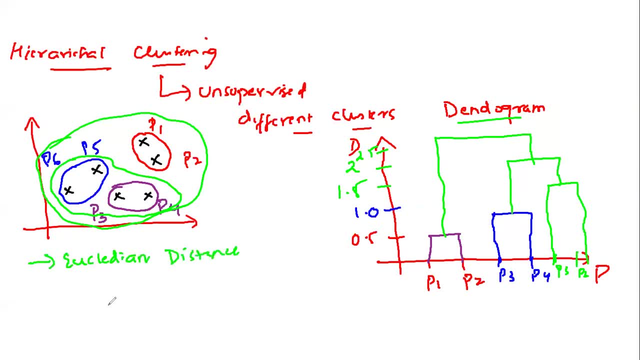 In my previous video also, I've discussed about Euclidean distance. This formula is basically given by: if I have two points- x1, y1 and x2, y2, I can give it by square root of x2 minus x3.. 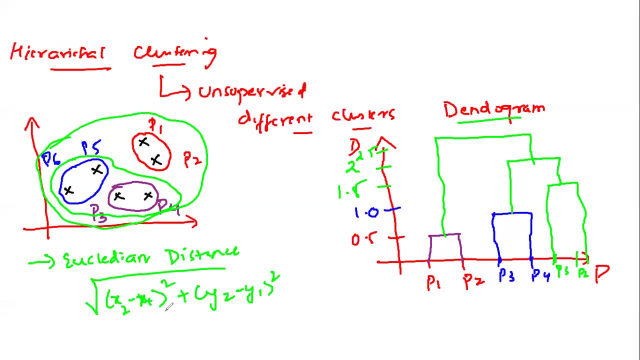 Square root of x2 minus x1 whole square, plus y2 minus y1 whole square. So this will be the distance between two points, P1 and P2, which is represented by x1, y1 and x2, y2.. Now the next thing is that how can I find out the number of exact clusters that I need to classify this problem? 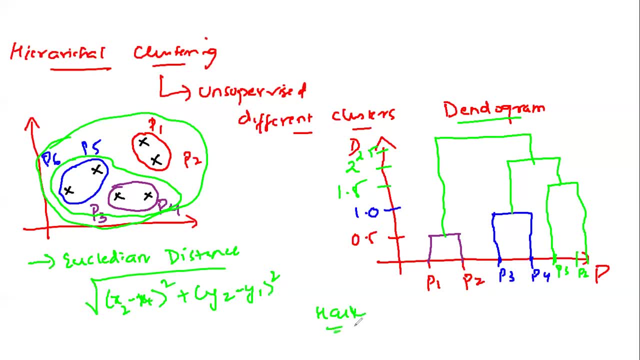 So there is a simple hack that is used. This hack is nothing. that we need to find out how many groups. We need to find out the longest vertical line, such that none of the horizontal line passes through. So I can't consider this particular line. 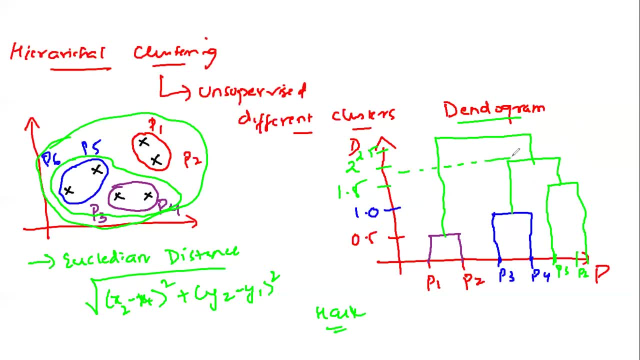 Because there is a horizontal line that passes through this particular point. Similarly, I can't consider this line, also because there is a horizontal line passing through this point. So, similarly, I can't consider this. I can't consider this. I can't consider this, also because there is a horizontal line passing through it. 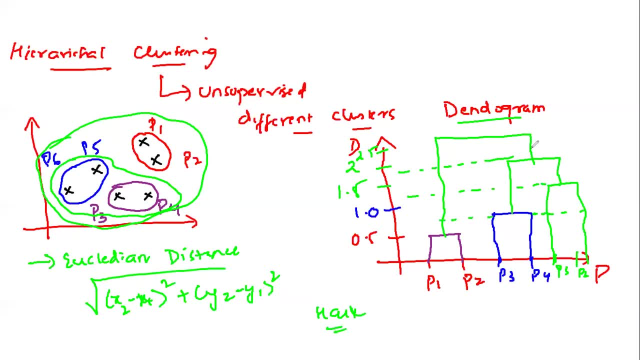 Now I can consider this particular line, because this may be the longest line compared to all the others. So what I do is that I'll draw a straight line that passes through this particular point, And I'll try to see how many points it is passing through. 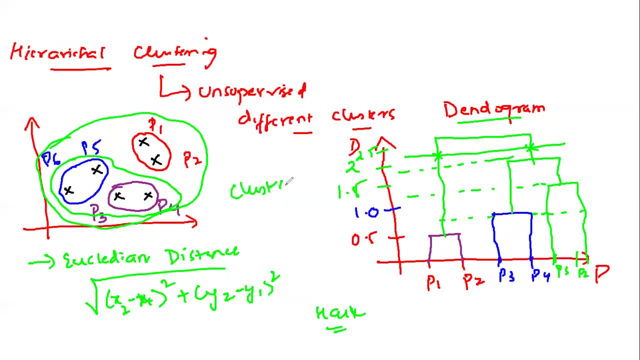 So there are two points that it is passing through, So I can specify that the number of clusters that I can use for this problem is basically 2.. And this is the hack basically used for the new one, And this is just a rough diagram. 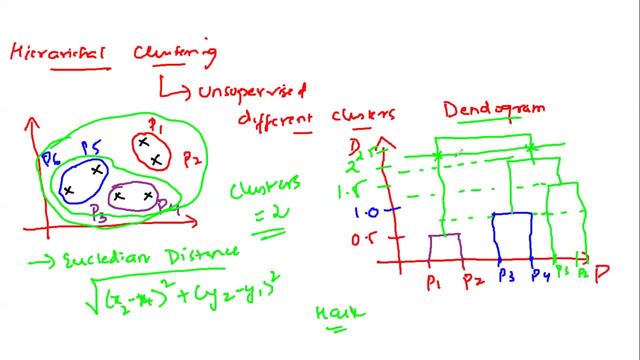 Your clusters may also get changed to 3. That depends on how many points it is passing. as soon as I find out the longest vertical line, And once I'm able to do this, I'll use an sklearn and try to use this hierarchical clustering.